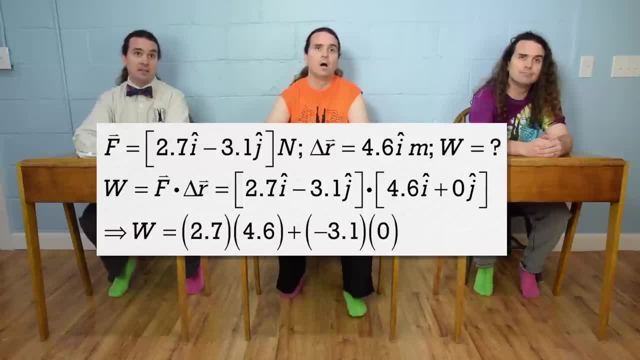 Multiply the i's together, multiply the j's together and take the sum, So it is 2.7 times 4.6, plus the negative 3.1 times 0 or 12.42, which is 12 with two significant digits. 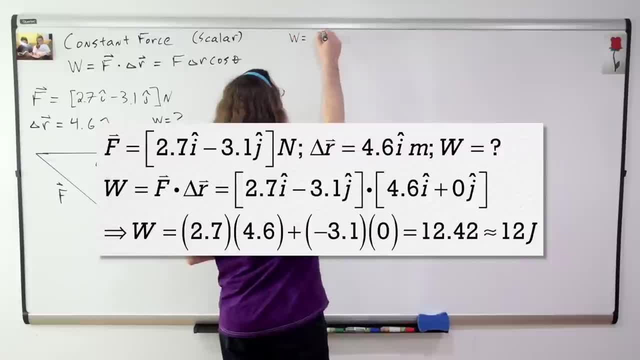 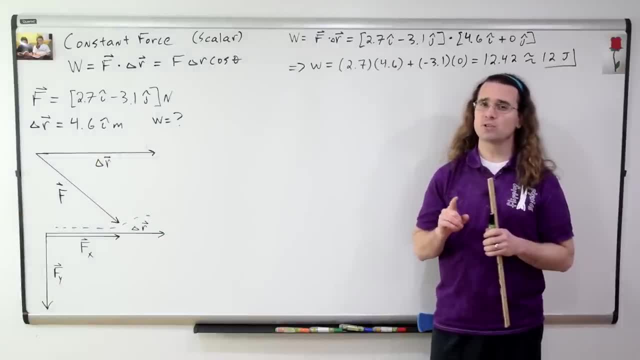 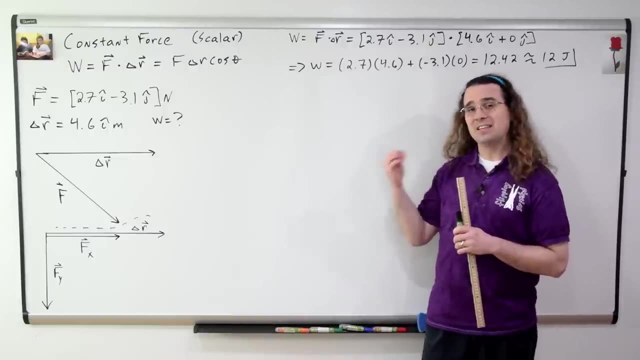 Okay, Oh, and it's in joules, Notice. the dot product multiplies the component of the force which is in the direction of the displacement of the object with the displacement of the object. In this particular case, the component in the direction of the displacement of the object is 2.7 newtons. 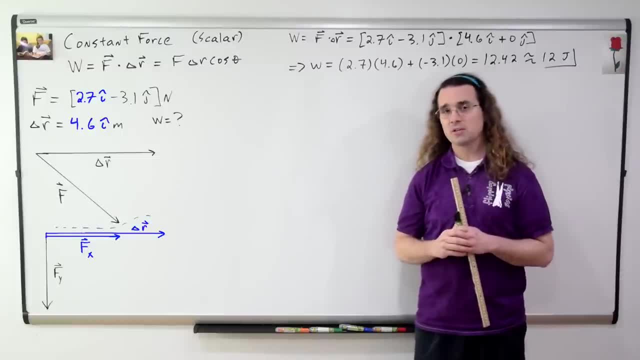 multiplied by the displacement of the object of 4.6 meters, The component normal to the direction of the displacement, in this particular case 3.1 newtons in the negative y direction, does no work on the object, again, because it is at a 90 degree angle to the displacement of the object. 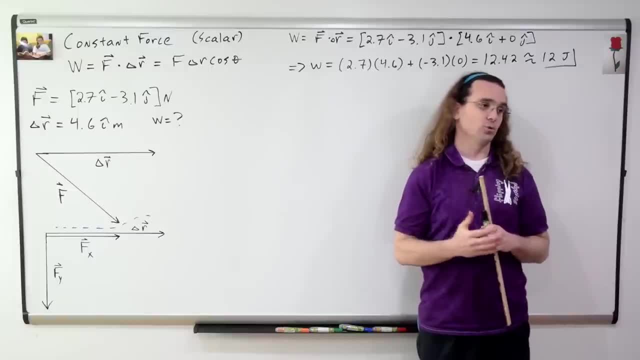 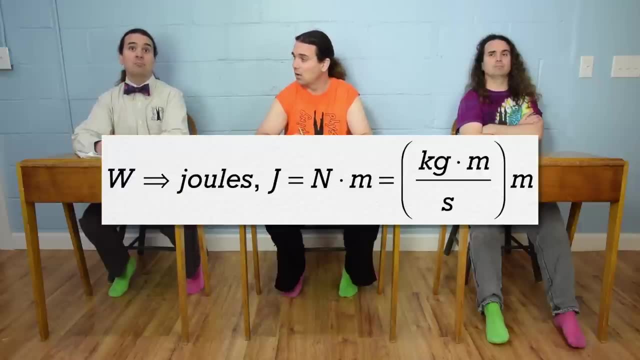 And yes, Billy, the units for work are joules. Bobby, what is a joule? A joule is a newton times a meter, And a newton is a kilogram meter per second Squared. Oh yeah, Kilogram, A newton is a kilogram meter per second squared. 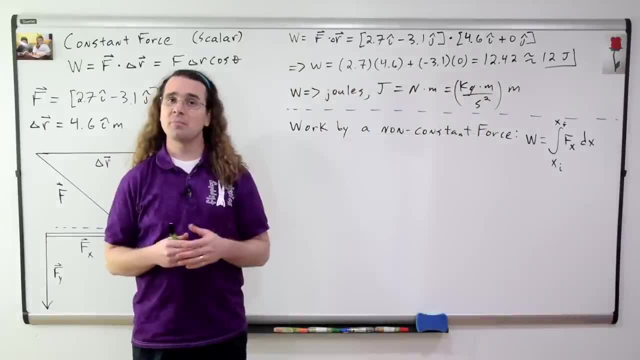 Okay, The work done by a force which is not constant uses a different equation. That work is equal to the integral from position initial to position final of the force with respect to position, And this is called a definite integral, Which simply means the integral has limits. 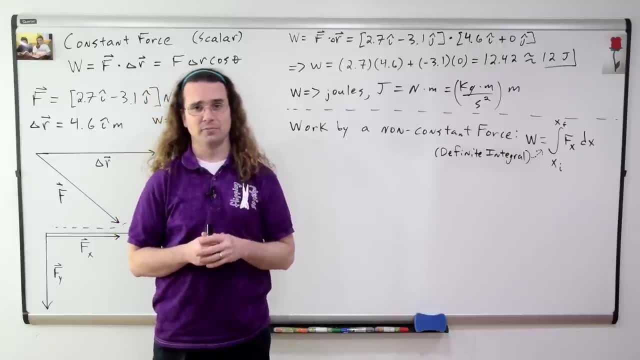 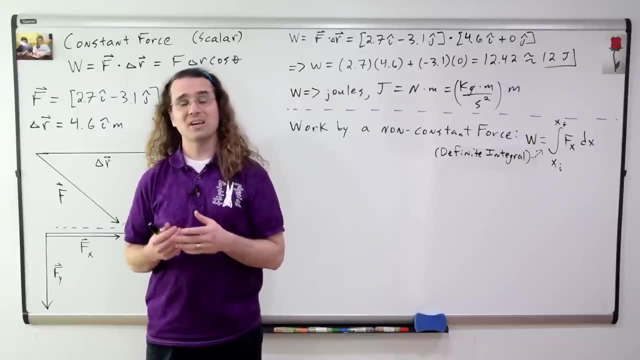 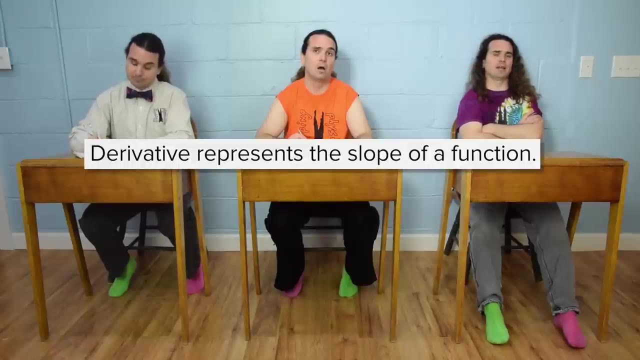 In this particular case, from the initial position to the final position Bo. the derivative represents the slope of a function. What does the integral or what we also call the antiderivative, represent? An integral or antiderivative represents the area under the curve. 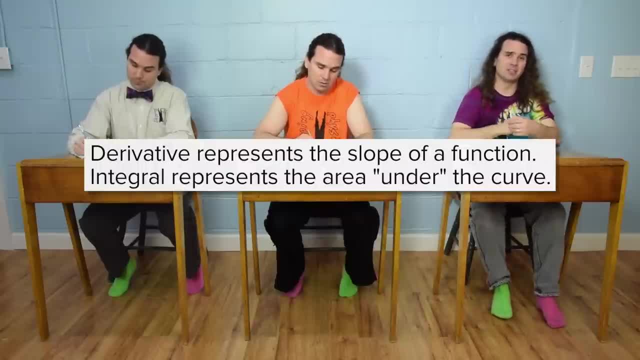 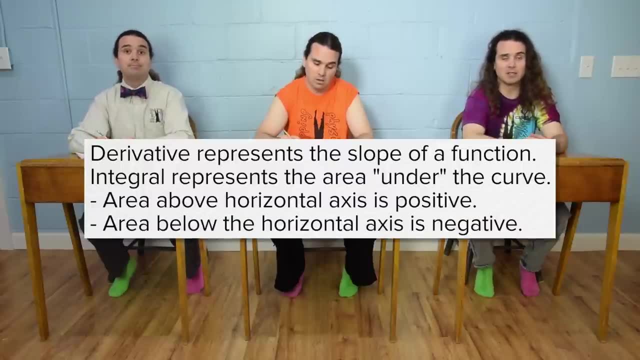 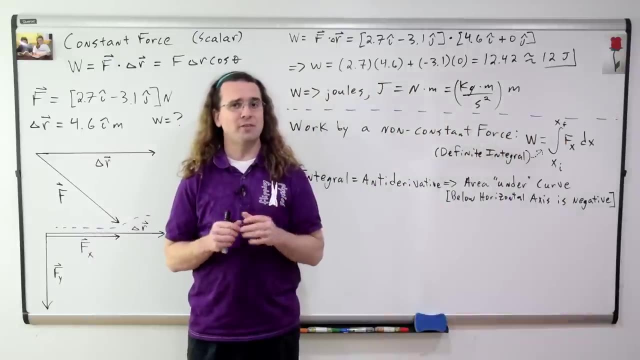 And the area under the curve means the area between the curve and the horizontal axis, And area above the horizontal axis is positive, Area below the horizontal axis is negative. Notice how we have two different equations for work. We use one equation for work when the force is constant. 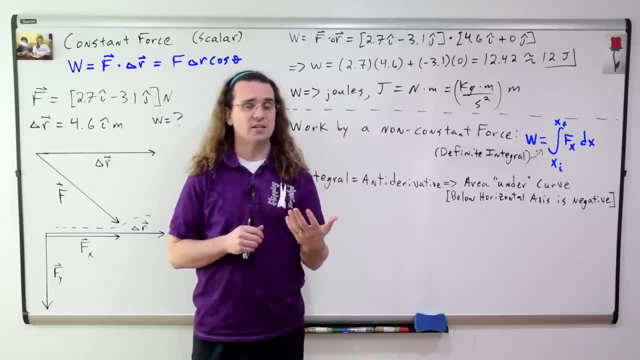 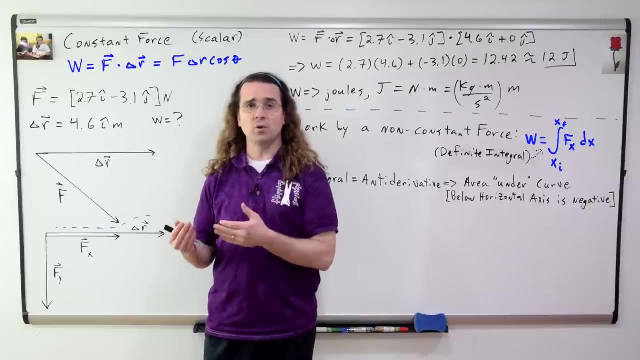 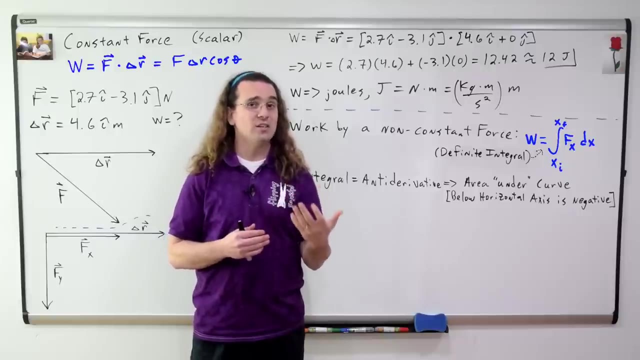 And we use a different equation for work when the force is not constant And that equation uses an integral. This is going to happen a lot in this class, Where we use one equation when the item does not vary And we use a different equation for that same item when that does vary. 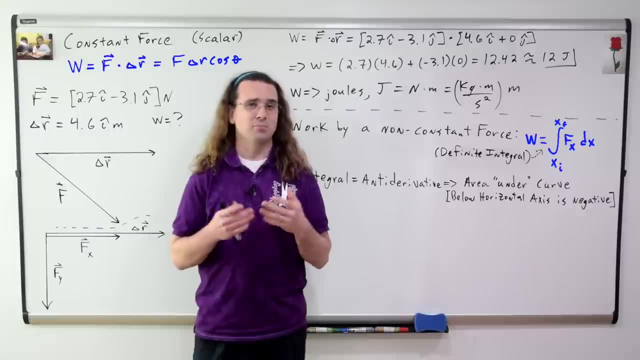 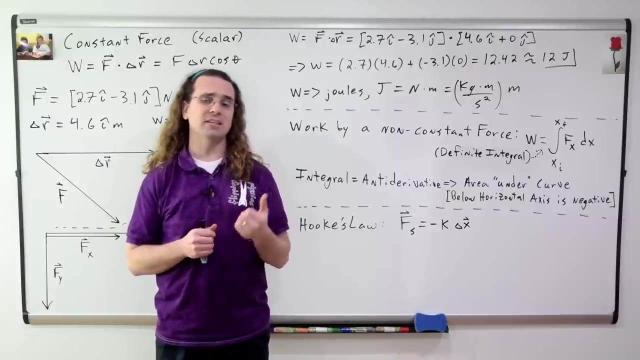 And that equation uses an integral, And please pay attention to that. Alright, now let's talk about the force caused by a spring. Hooke's Law: The force of a spring equals negative kx. Bobby, could you please clarify all of these letters? 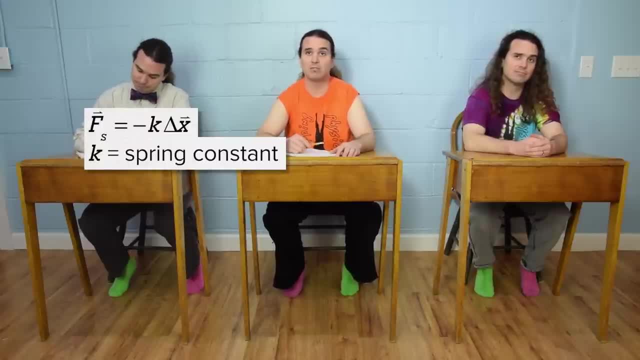 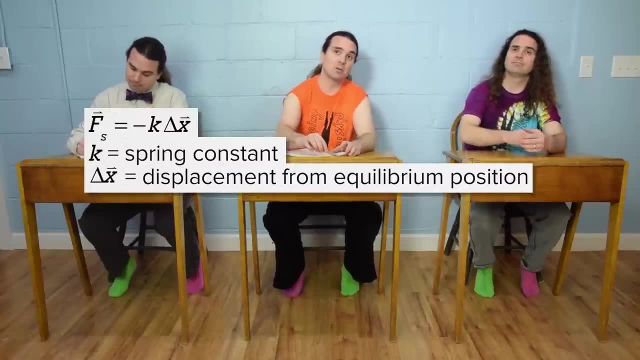 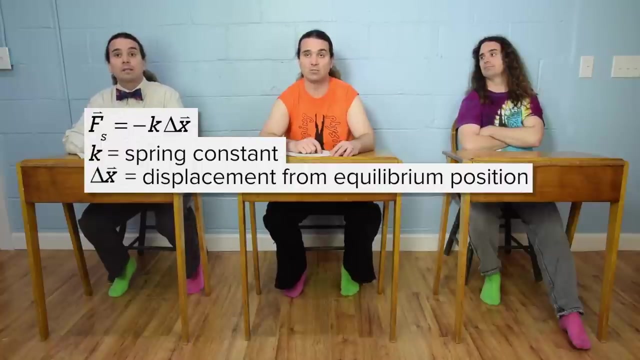 k is the spring constant And it is a measure of how much force it takes to compress or expand the spring per meter. Delta x is the displacement of the spring from equilibrium position or rest position, which is where the spring would be if it were not being compressed or elongated. 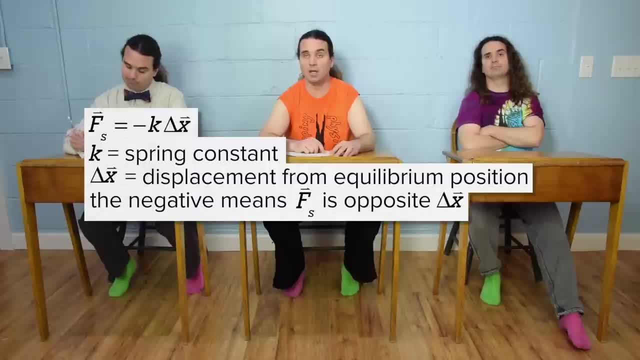 The negative has to do with the direction of the force of the spring. It means the force of the spring is opposite the direction of the displacement of the spring, And the units for the spring constant are usually newton meters. Actually it's newtons per meter. 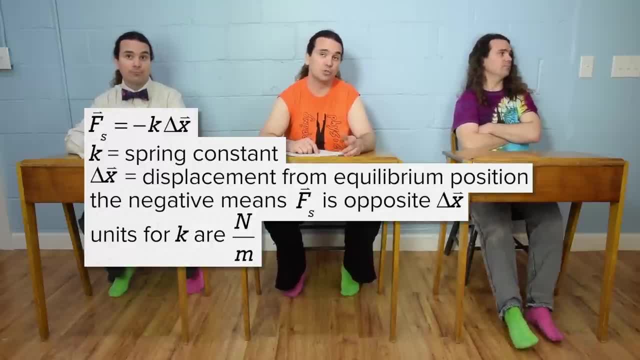 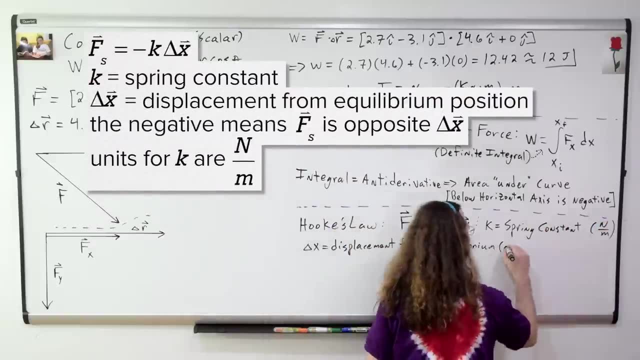 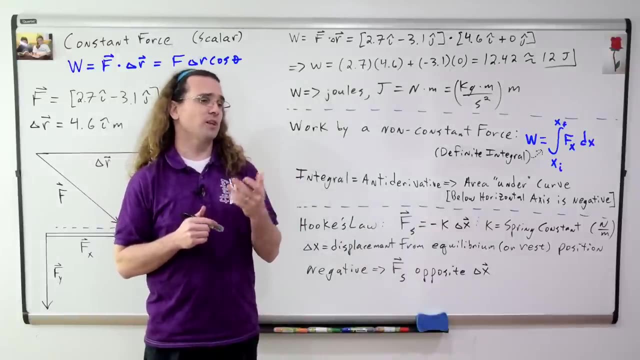 The spring constant is in newtons per meter. Joules are newtons times meters. Thanks, I always mess that up. You are welcome, Billy. which of the two work equations do we use when determining the work done by the force of a spring? Well, that would depend on whether the force caused by a spring is constant or varies. The force caused by a spring changes with position, so it is not constant, Right. Therefore, the work done by a spring equals the integral from position initial to position final. 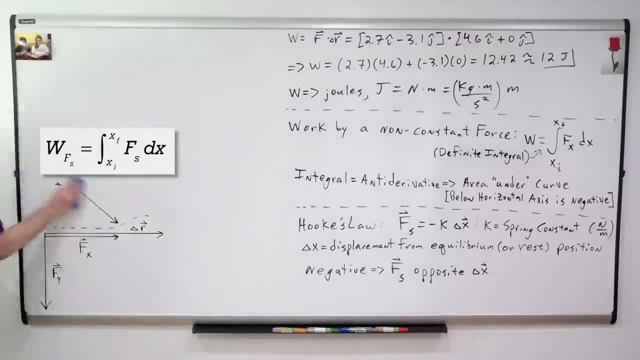 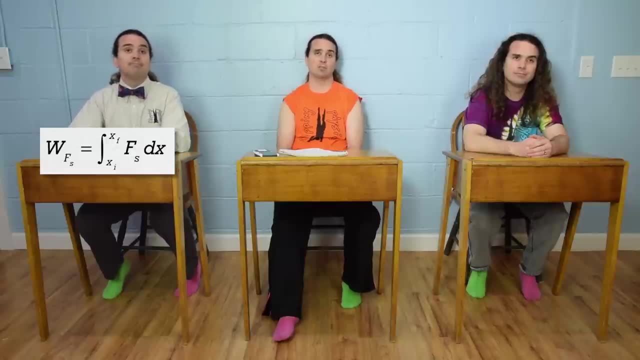 of the force of the spring with respect to position. Bobby, please determine the work done by a spring. Well, the equation for the spring force is the negative of the spring constant times, the displacement from equilibrium position. The integral of x to the first power with respect to x is x squared over 2.. 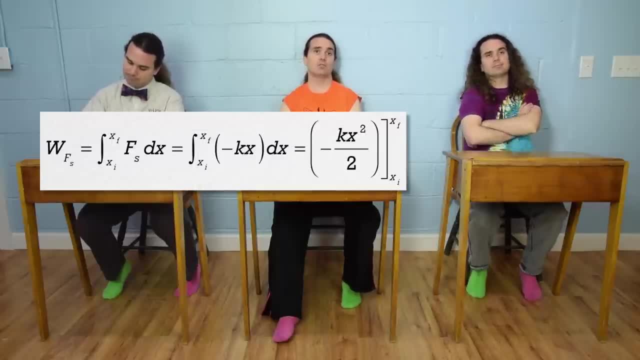 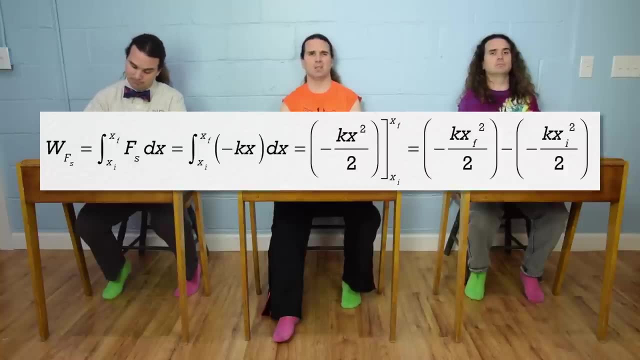 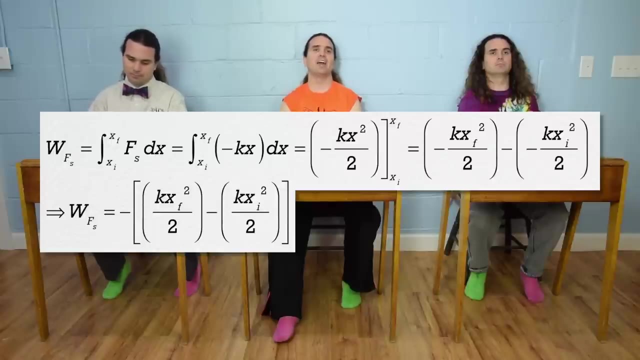 So we have negative kx squared over 2 from position initial to position final. Substituting in our limits gives us way too many negatives, So I'm going to factor out a negative 1.. And 1 half kx squared is elastic potential energy. 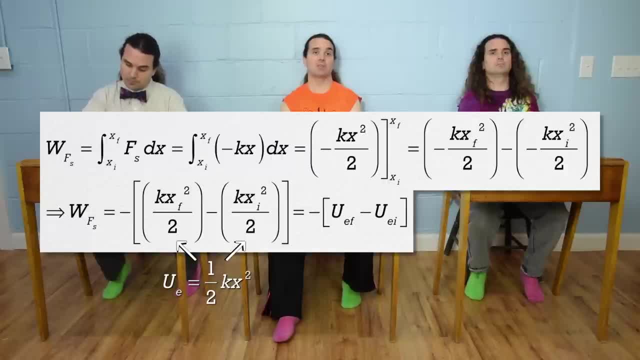 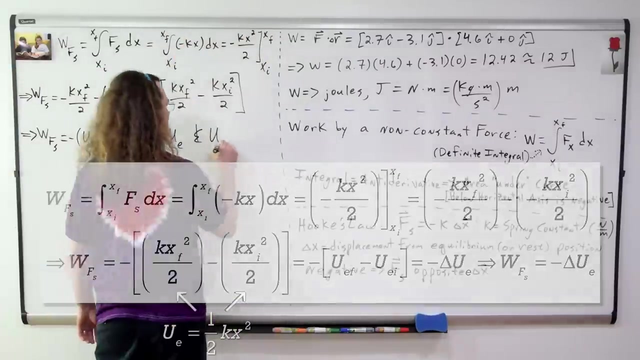 So that is the negative of elastic potential energy final minus elastic potential energy initial, or the negative of the change in elastic potential energy of the spring. The work done by a spring force equals the negative of the change in elastic potential energy of the spring. That's pretty cool. 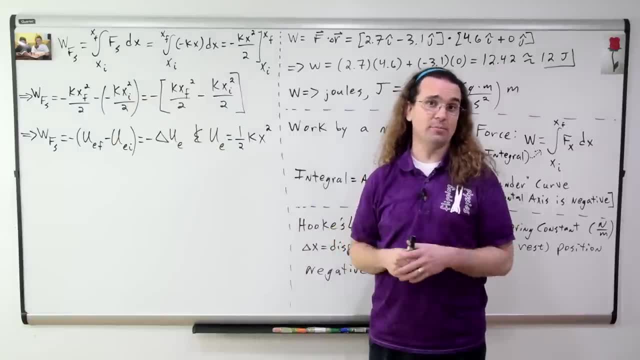 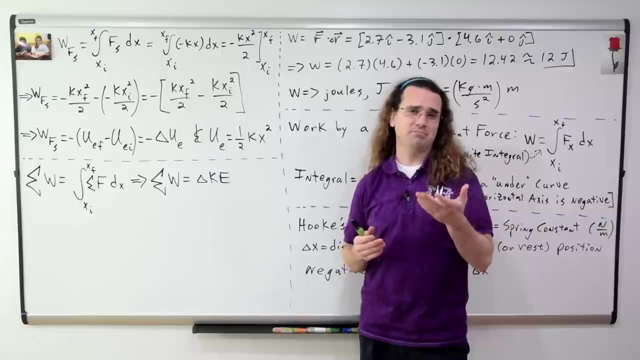 Previously we derived the network kinetic energy theorem. We're not going to do that derivation right now. However, you're more than welcome to review it by clicking on the link which just appeared. It was during that derivation where we defined kinetic energy. 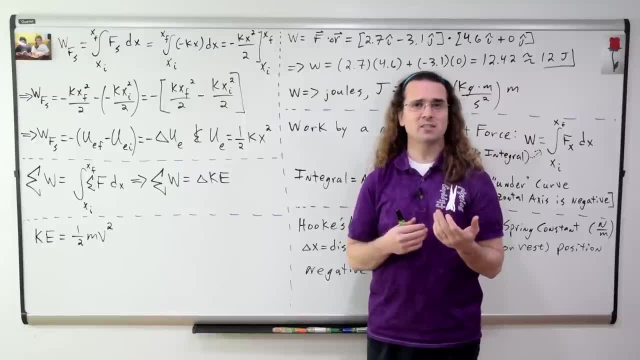 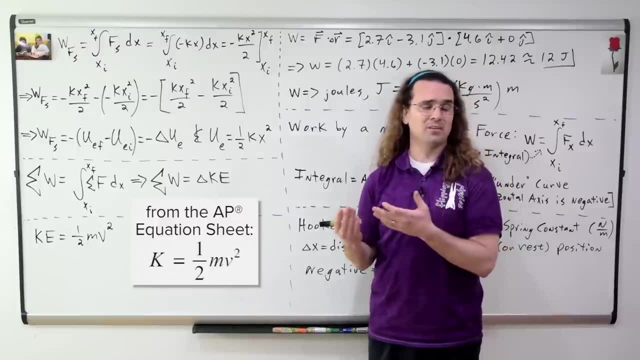 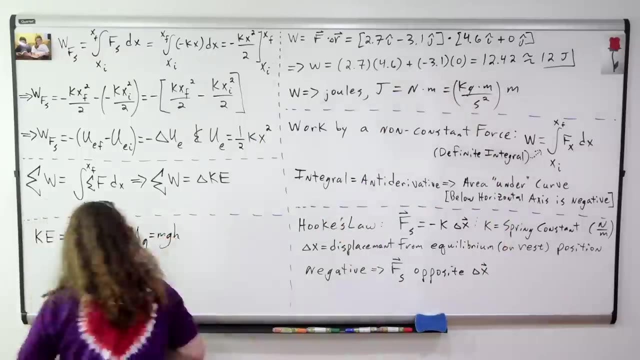 Kinetic energy equals 1 half times the mass of the object times the velocity of the object squared. The AP equation sheet just uses the capital letter K. I prefer capital KE so that you don't confuse the spring constant with kinetic energy. Gravitational potential energy equals the mass of the object. 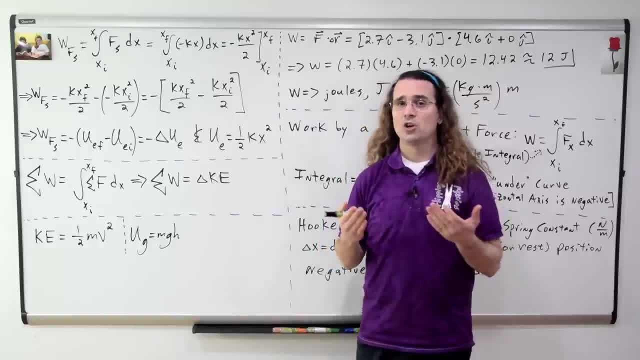 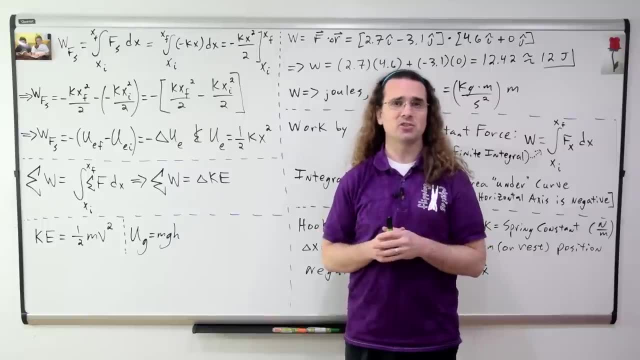 times the acceleration due to gravity. times h the vertical height above the horizontal zero line. And please don't ask me why the symbol for gravitational potential energy is a capital U. I don't know. Please remember whenever you use gravitational potential energy. 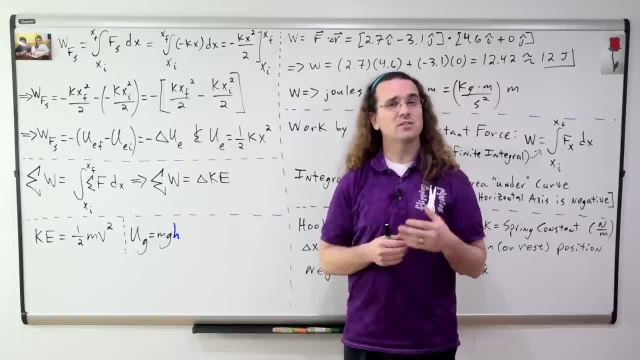 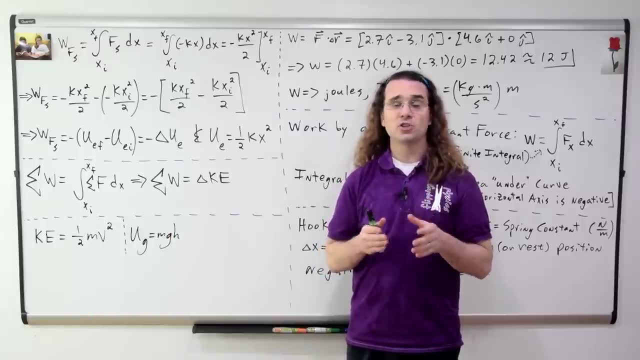 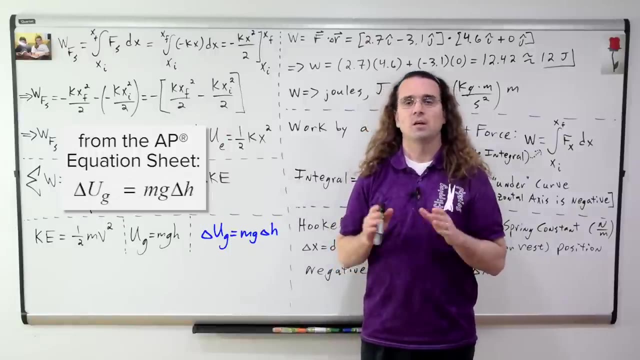 you have to identify the horizontal zero line. This is the reference line for the vertical height h. Now the equation on the AP equation sheet is instead in terms of the change in gravitational potential energy. Okay, energy can neither be created nor can it be destroyed. 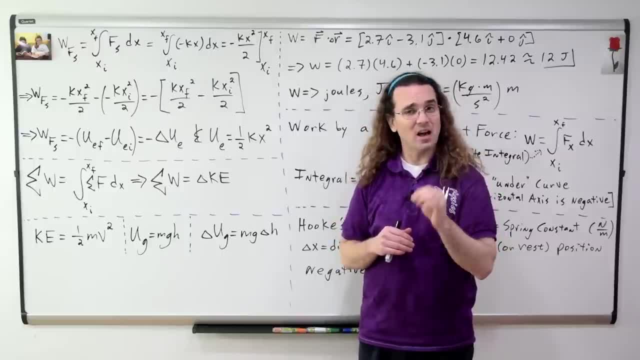 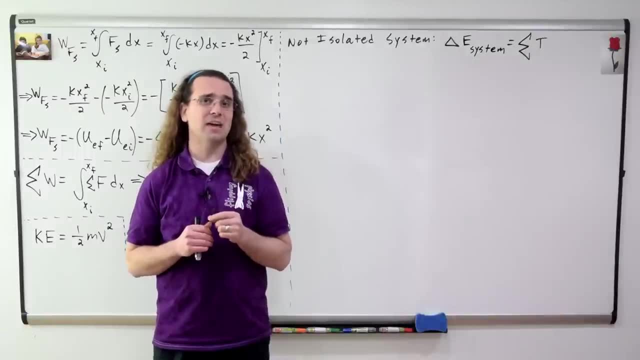 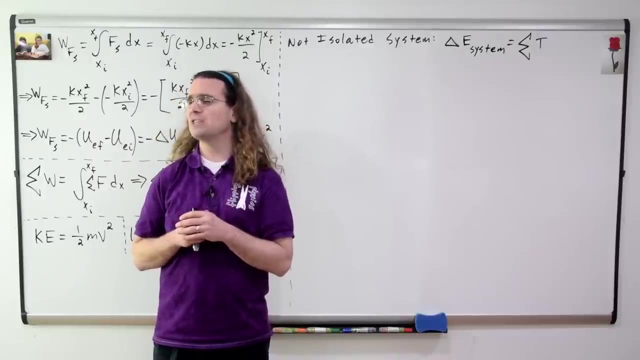 Therefore, in a system which is not isolated, the change in energy of the system equals the sum of the energy which is transferred into or out of the system Bo. this is important. Could you please review it for us? Sure, When we have a non-isolated system, 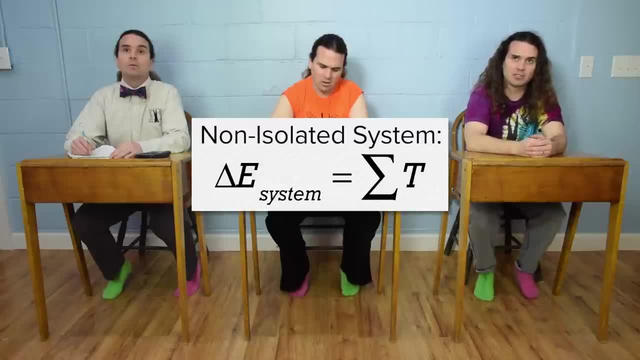 which means a system which is receiving energy or having energy taken away from it. the change in energy of the system equals the addition of all the energy which is transferred into or out of the system. It actually makes a lot of sense if you think about it. 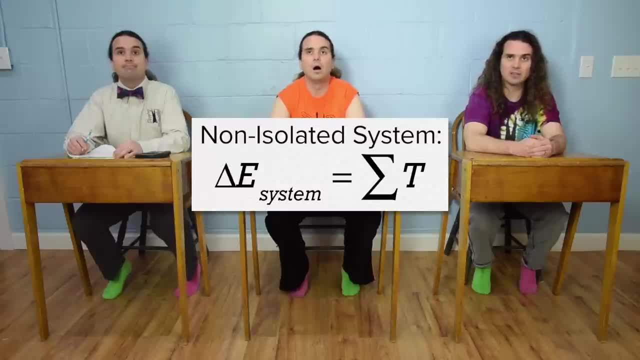 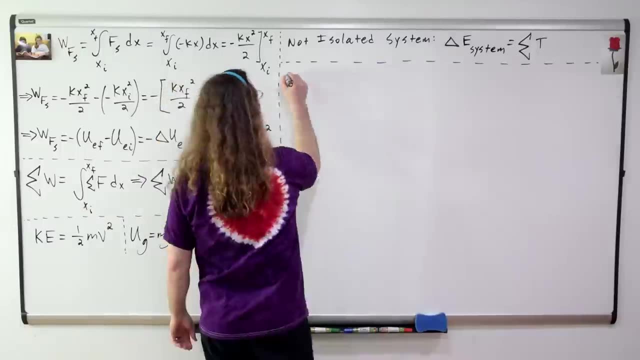 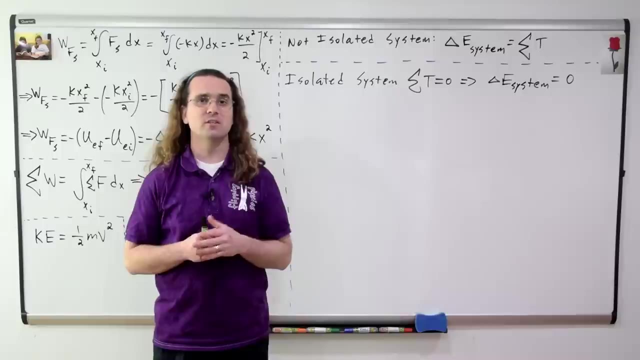 because you cannot create or destroy energy. The energy has to come from or go somewhere Right Now. if the system is isolated, then no energy is transferred into or out of the system. Therefore, the change in energy of the system must be zero. 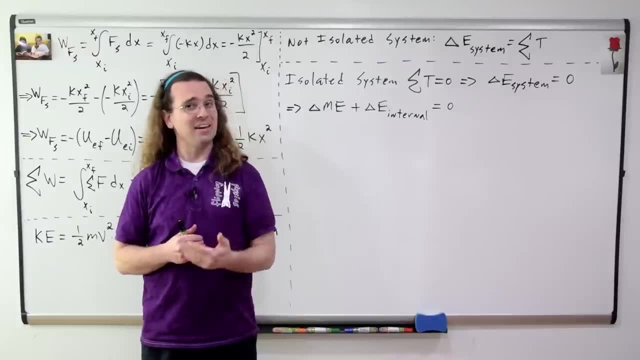 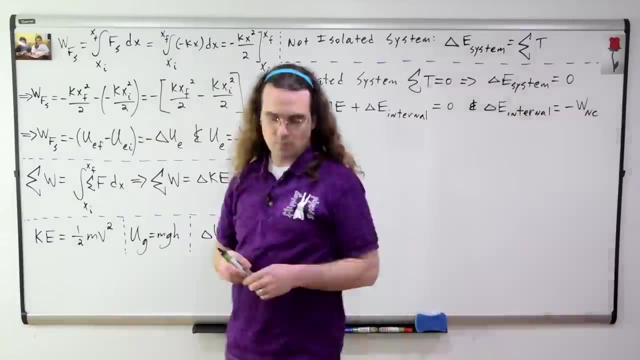 The change in energy of the system equals the change in mechanical energy of the system plus the change in internal energy of the system, which add up to zero. The change in internal energy of the system equals the negative of the work done by non-conservative forces. 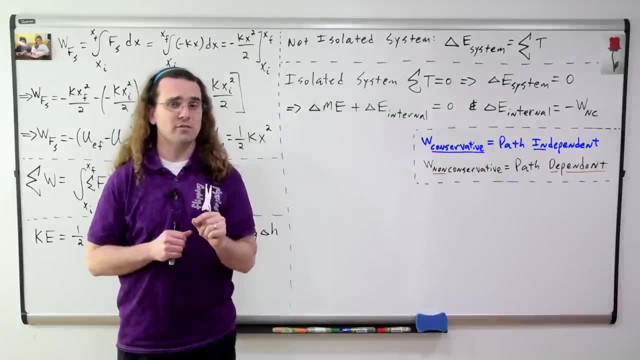 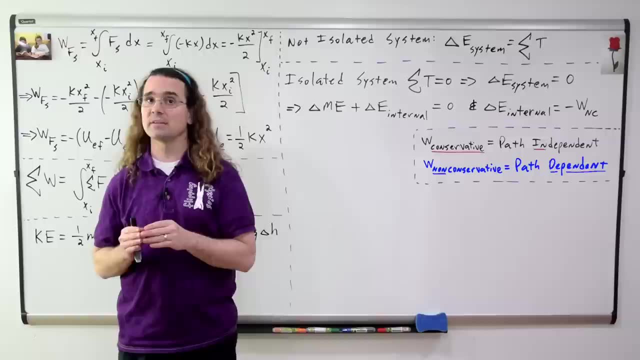 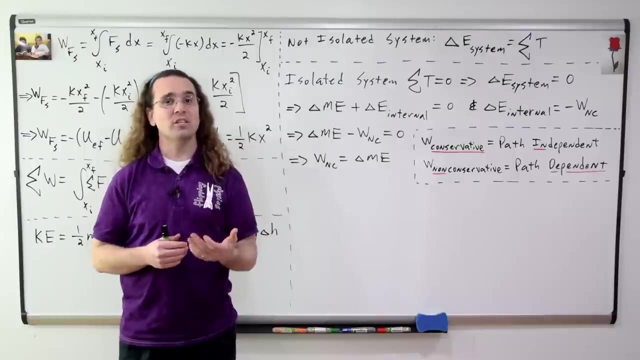 And remember, the work done by a conservative force does not depend on the path taken by the object and the work done by a non-conservative force does depend on the path taken by the object. Therefore, the work done by non-conservative forces, 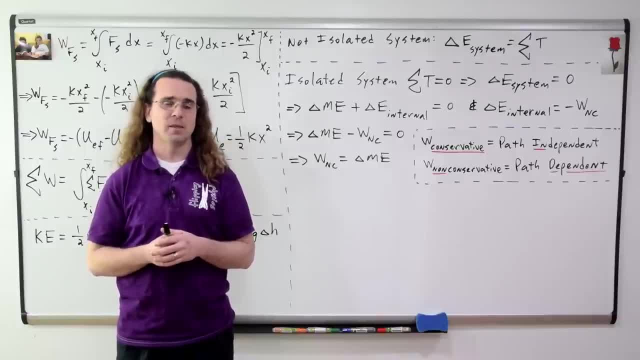 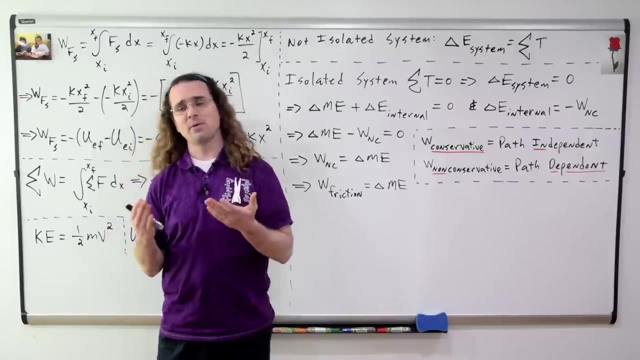 equals the change in mechanical energy of the system. And because the only non-conservative force that I know of is friction, I usually write this equation as the work due to friction equals the change in mechanical energy of the system. And remind me, Bobby, what needs to be true. 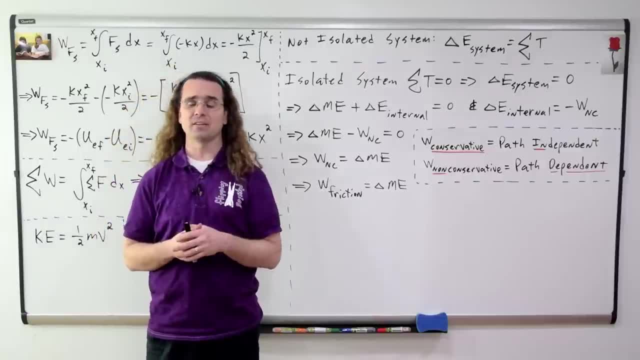 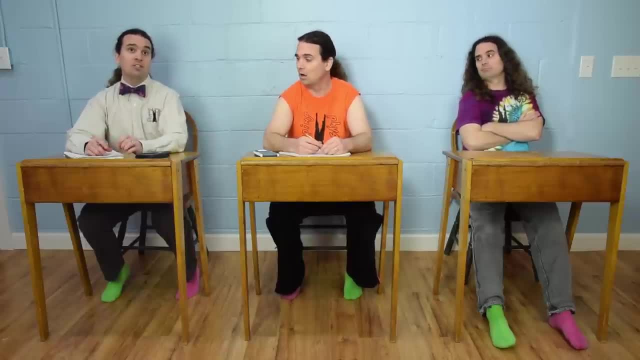 for the work due to friction to be equal to the change in mechanical energy of the system, There needs to be no energy transferred into or out of the system. The system needs to be isolated Right And don't confuse the work due to friction. 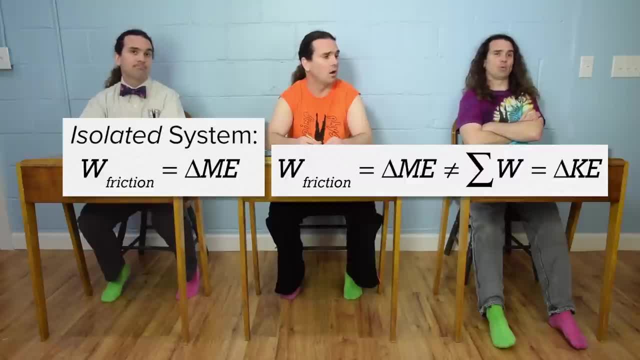 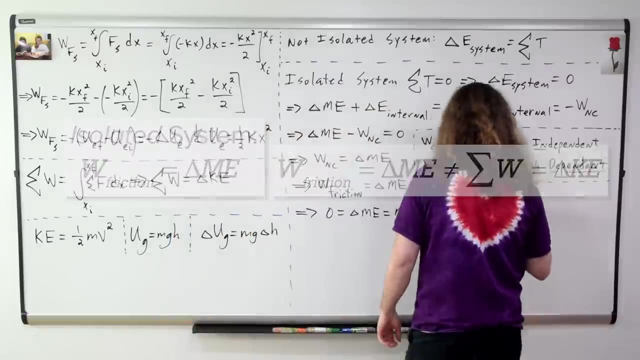 equals change in mechanical energy equation, with the network. equals change in kinetic energy equation. They do look similar, Right. Network equals change in mechanical energy is not the same as work due to non-conservative forces. equals change in mechanical energy. And if the system is isolated? 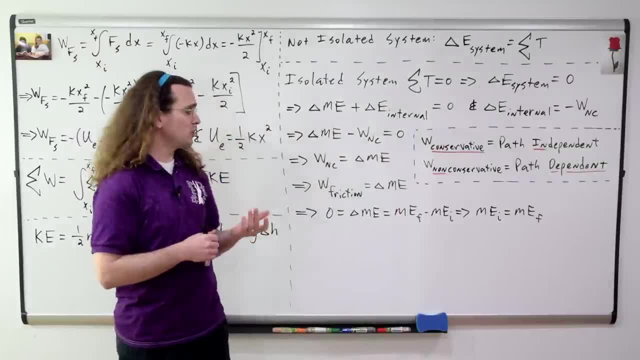 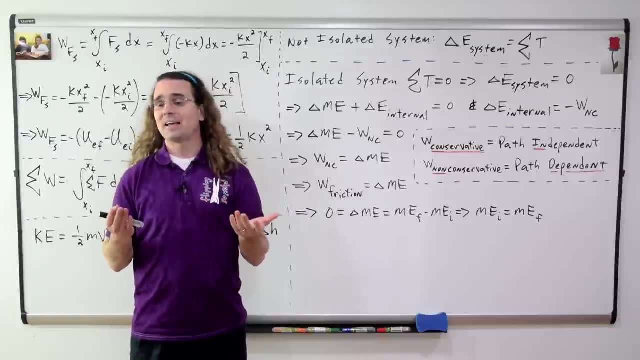 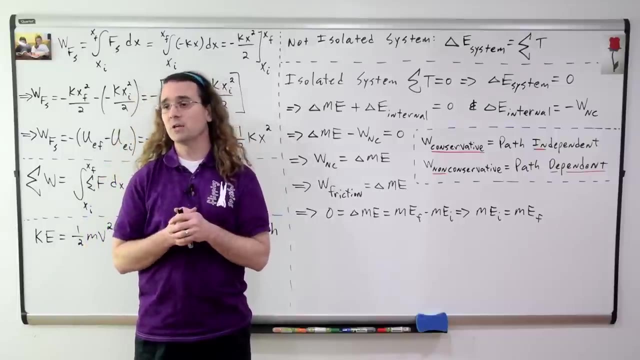 and no work is done by friction, then the change in mechanical energy equals zero, which works out to be conservation of mechanical energy. And class? remind me, what do you need to identify whenever you use? conservation of mechanical energy or work due to friction equals change in mechanical energy. 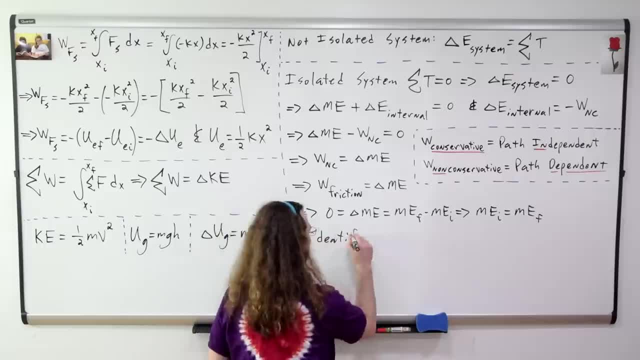 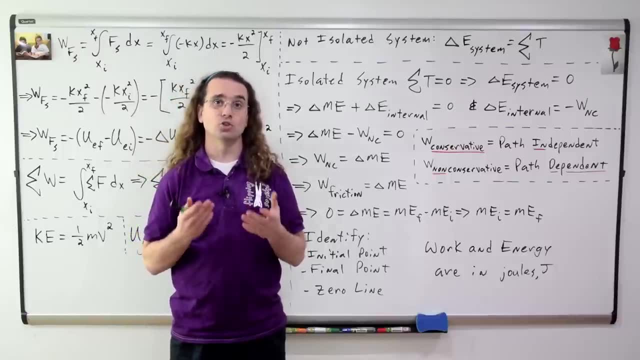 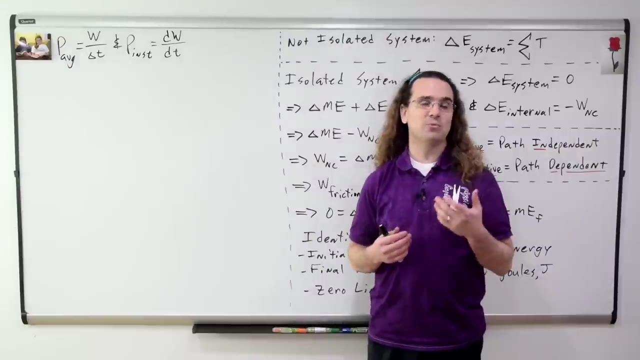 Initial point. Final point, Horizontal zero line. Remember, just like work, all of these forms of mechanical energy are in joules. Now let's talk about power. Power is the rate at which work is done. Therefore, average power equals work over change in time. 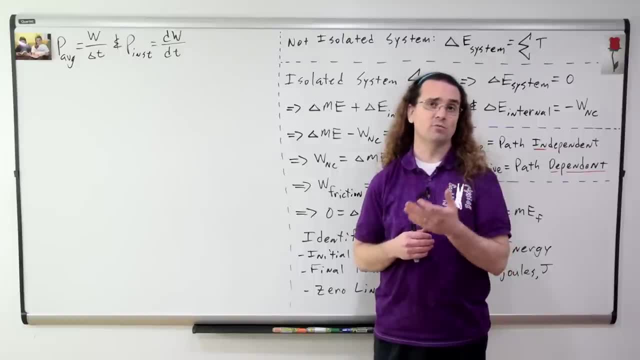 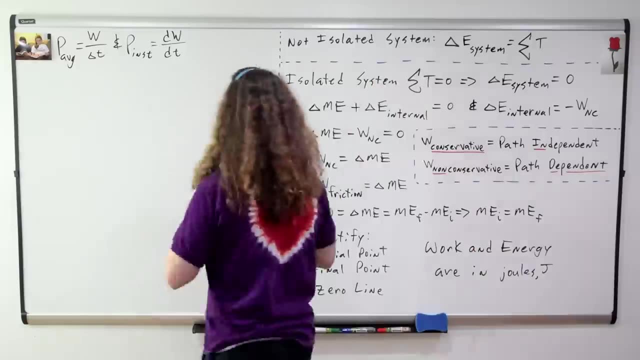 and instantaneous. power equals the derivative of work with respect to time. And I will point out that the equation for power in terms of work on the AP equation sheet is: power equals the derivative of energy with respect to time. Okay, Now substituting in the equation: 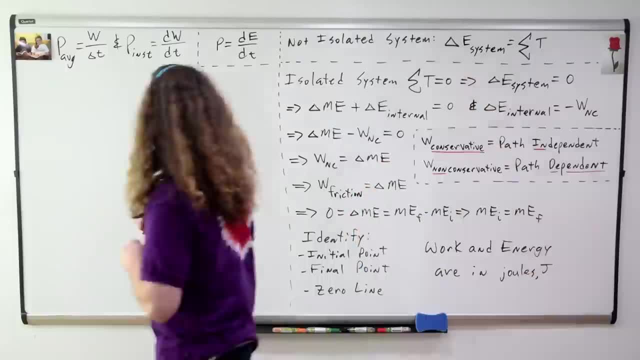 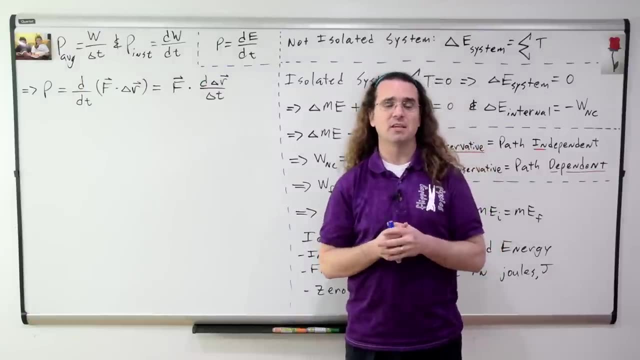 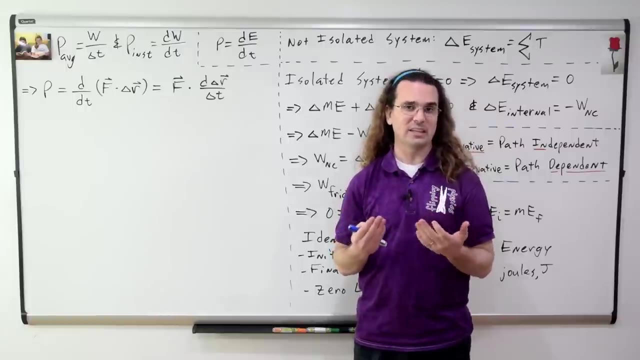 for work done by a constant force gives us the derivative, with respect to time, of the dot product of the force and the displacement of the object. But the force is constant, so this is really just the derivative of the position with respect to time, which is velocity. 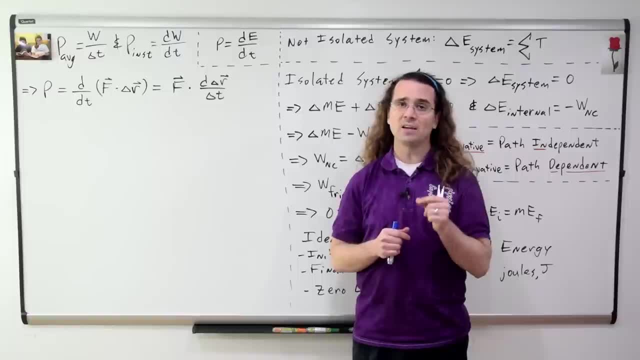 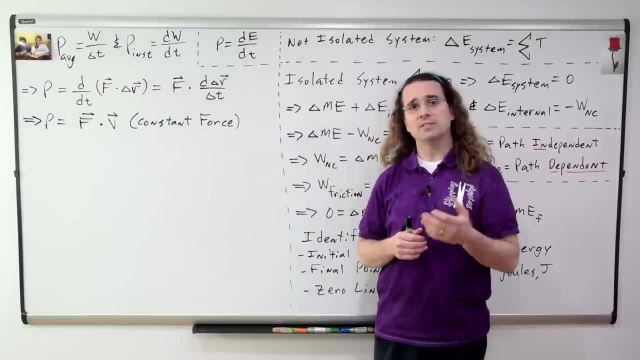 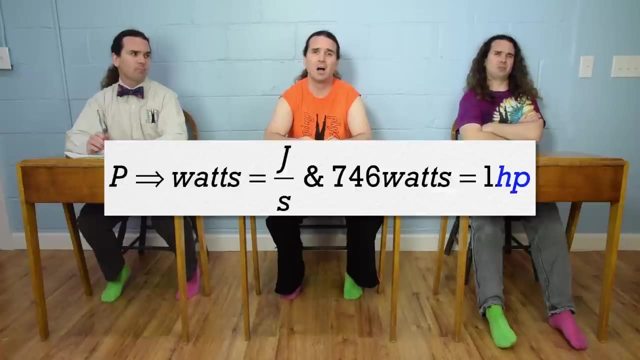 Therefore, the power delivered by a constant force on an object in terms of velocity is the dot product of force and velocity, Bo. what are the SI units for power? Power is in horsepower. Horsepower is the English unit for power. Watts are the SI unit for power. 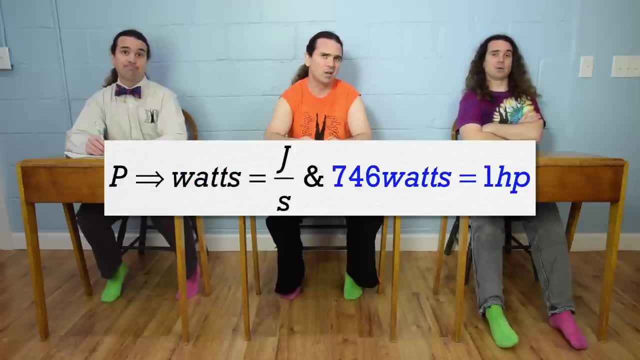 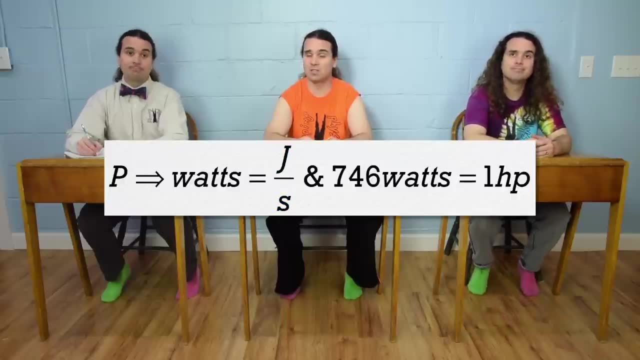 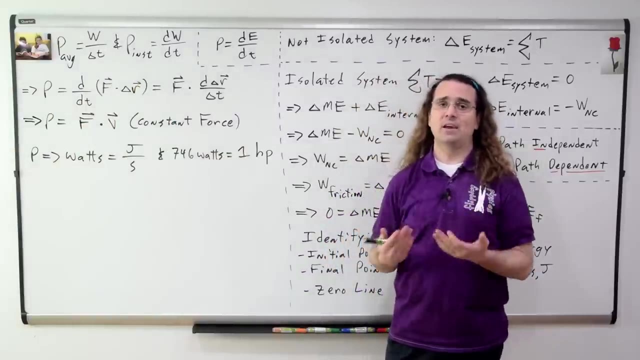 Right, and 746 watts equals one horsepower And watts are joules per second. But we don't have to memorize that there are 746 watts in one horsepower, right? You are correct that you do not need to remember how many watts are in a horsepower. 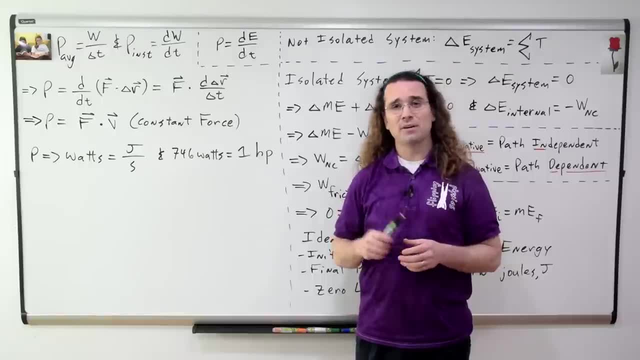 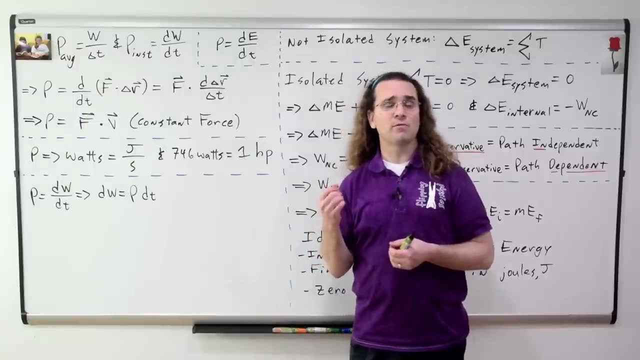 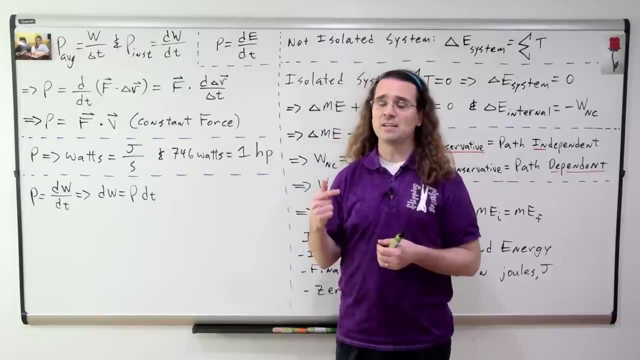 What you do need to remember is that every derivative is an integral or an antiderivative. For example, power equals the derivative of work. with respect to time can be rearranged to: dw equals power times dt. Taking the definite integral of both sides gives the change in work equals the integral. 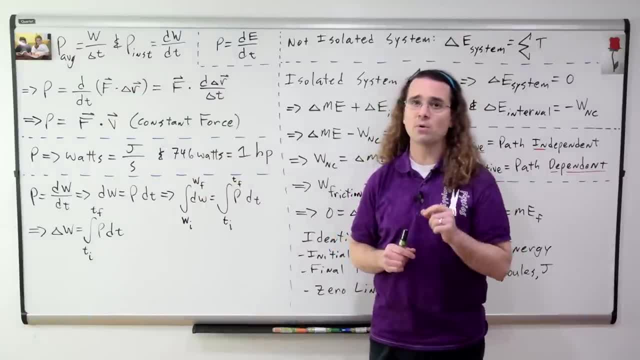 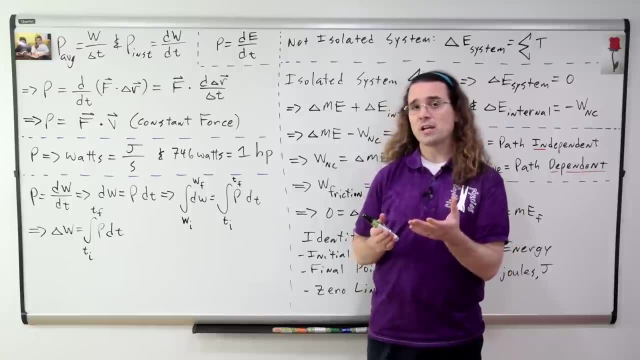 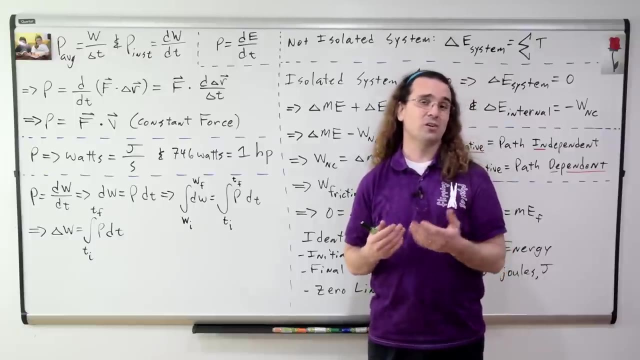 from time initial to time final of power with respect to time, Which means if you have a graph of the power exerted on an object with respect to time, the area under that curve will be equal to the change in work exerted on that object. 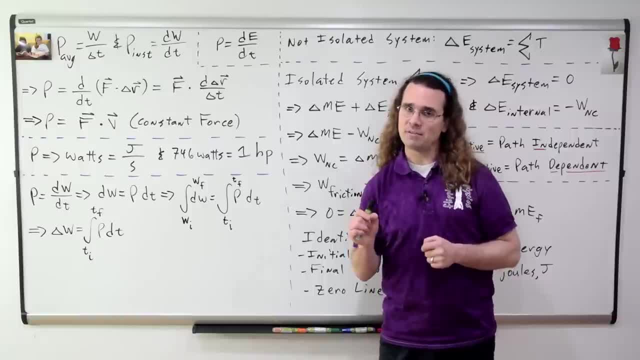 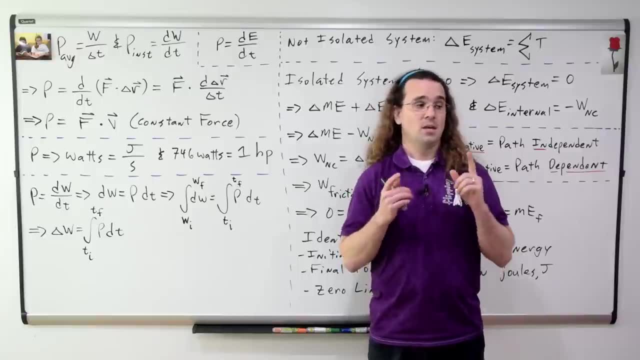 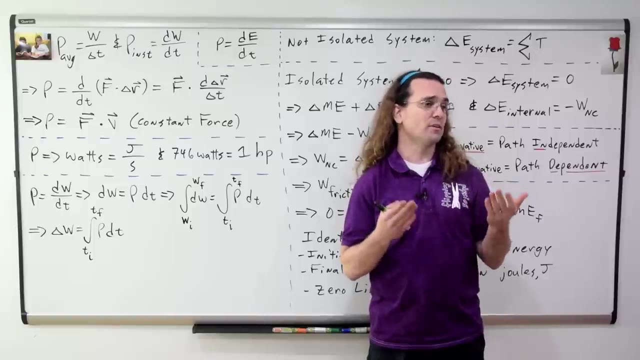 which could be very helpful. So please remember, every derivative can be rearranged as an integral and every integral can be rearranged as a derivative. Billy, what is the equation which is not on your AP equation sheet, which has to do with conservative forces? 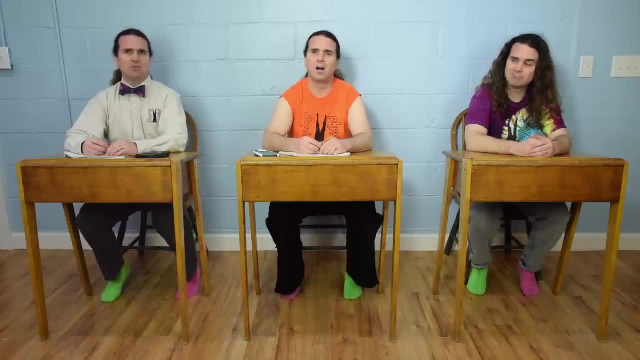 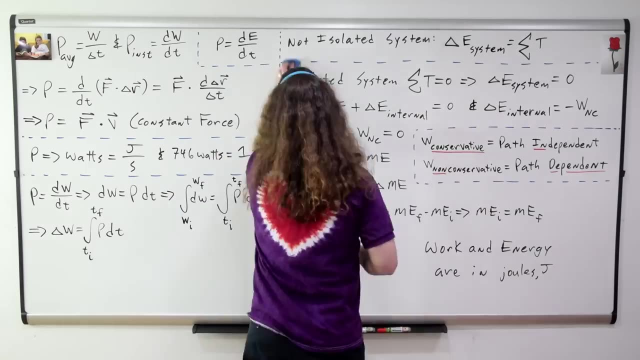 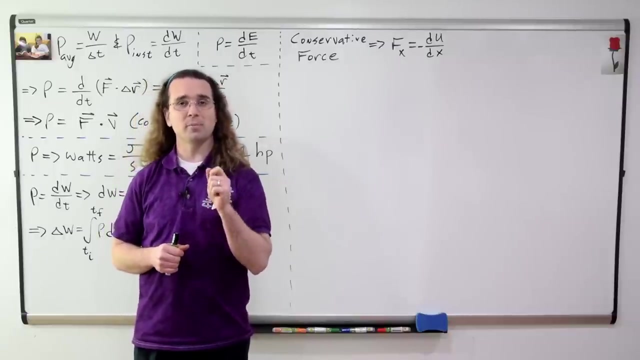 There is an equation which has to do with conservative forces which is not on our equation sheet. I do not know that, It's a pickle Pickle. A conservative force equals the negative of the derivative of the potential energy associated with that conservative force. 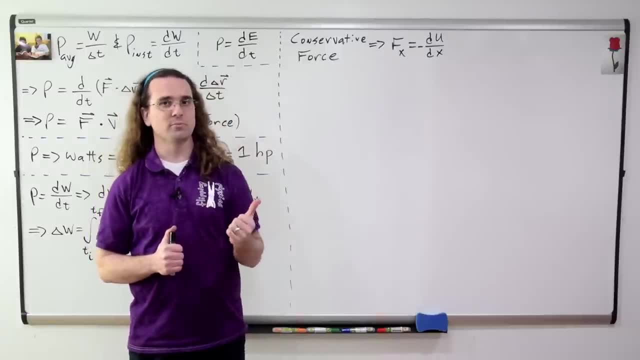 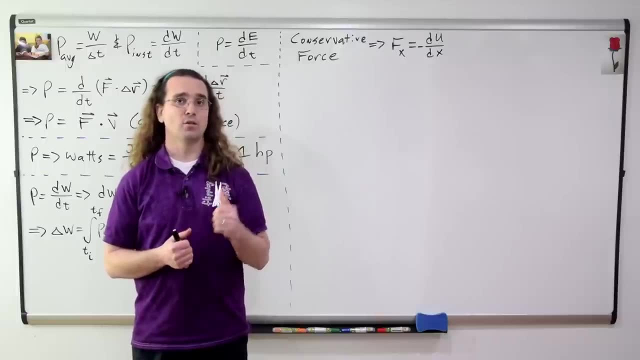 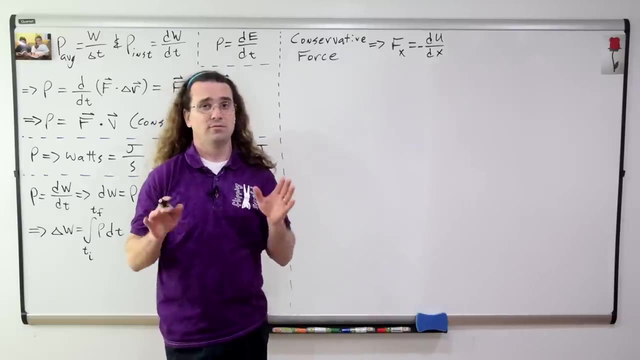 As a side note. you have to know this equation because much of the time when the phrase conservative force is used on the AP exam, this is the equation you need to use: Capisce Capisco, Ich verstehe, For example, for a spring. 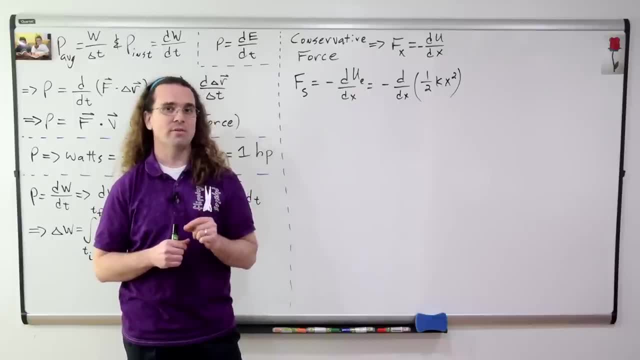 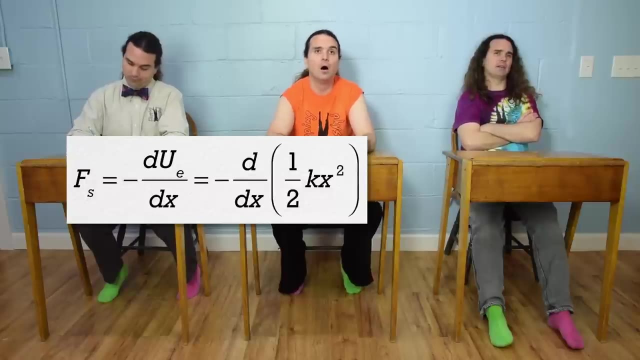 The force of a spring equals the negative of the derivative of the elastic potential energy associated with that spring with respect to position, And we can substitute in the equation for elastic potential energy And Bo. could you please take that derivative, The derivative of x squared with respect to x. 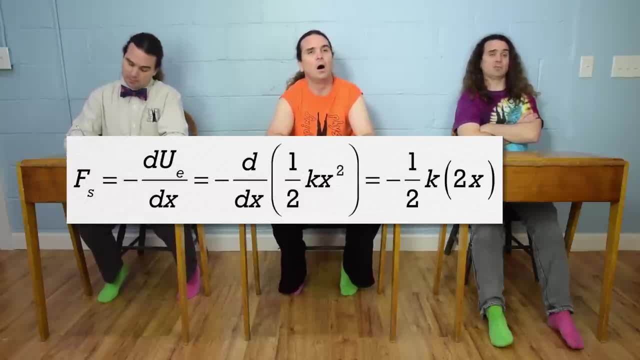 is 2 times x, And 1 half times 2 is 1.. So the force of a spring equals negative k times x. But we already know that, don't we Bo? that is my point, Right, Billy? could you please do the same thing? 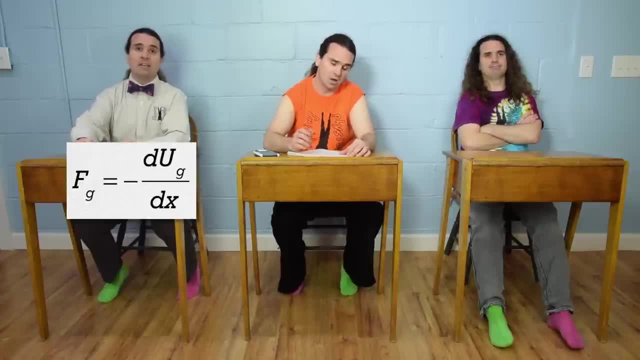 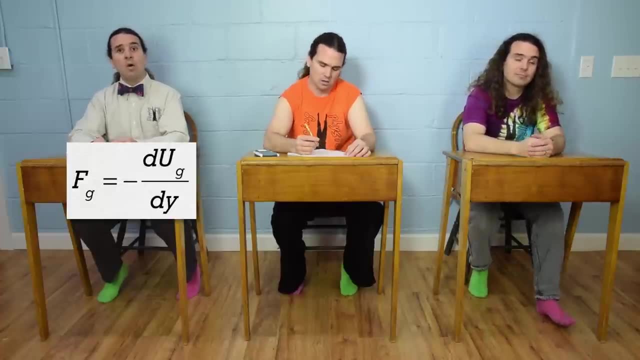 with the force of gravity. The force of gravity equals the negative of the derivative of gravitational potential energy with respect to position. However, that position is going to be in the y direction because the force of gravity is in the y direction For gravitational potential energy. 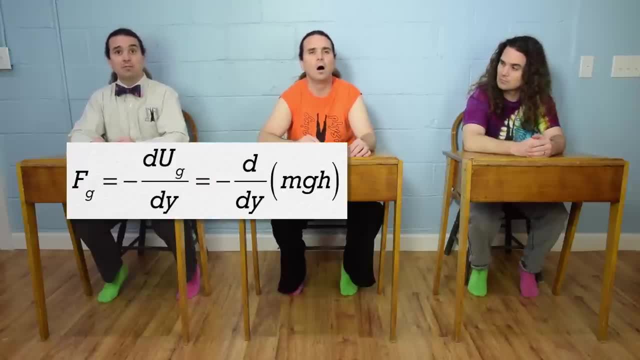 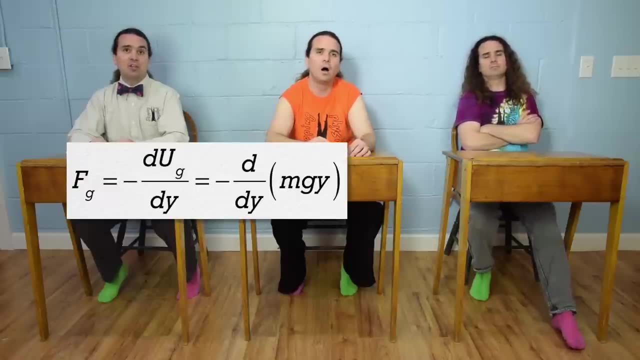 we can substitute in mass times acceleration due to gravity times, vertical height above the horizontal zero line, Although let's use y for that instead of an h, to match the variable we used for position. Mass and acceleration due to gravity are constants And the derivative of y with respect to y is just 1.. 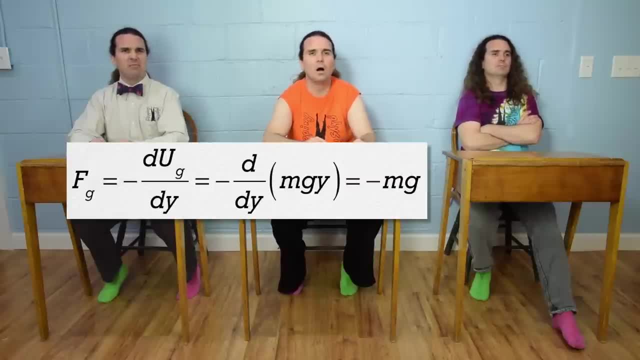 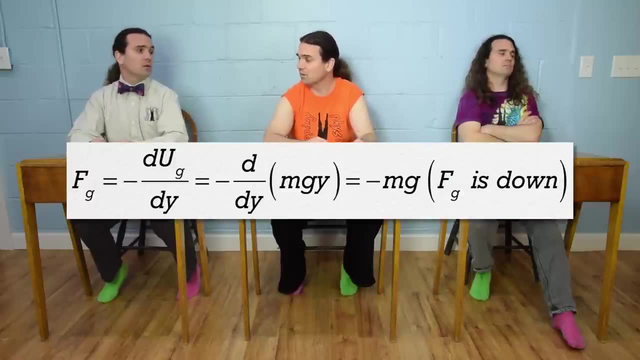 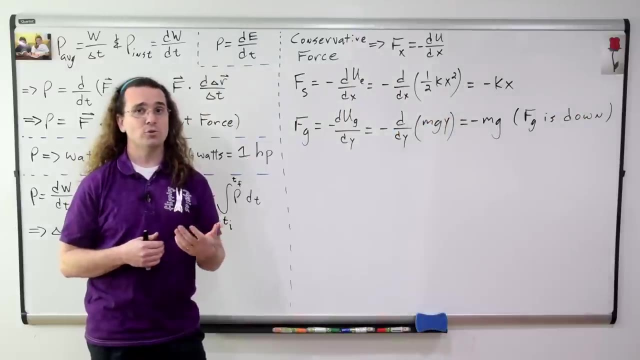 So the force of gravity equals the negative of mass times, acceleration due to gravity. Why is it negative? The force of gravity is always down. That's why it is negative. Okay, that makes sense. Now let's talk about neutral, stable and unstable equilibrium.